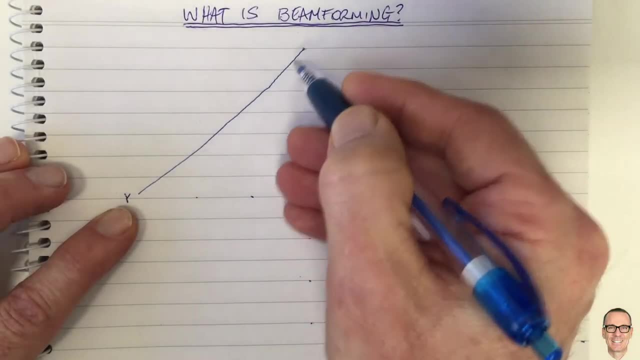 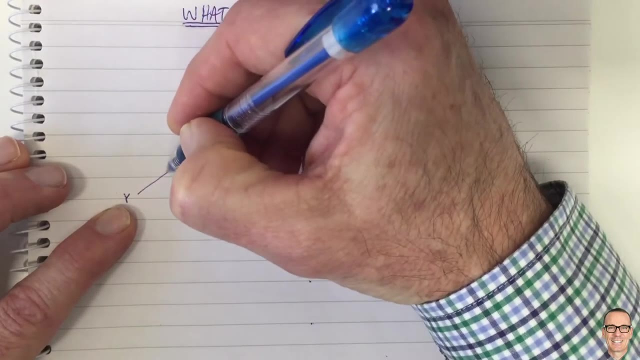 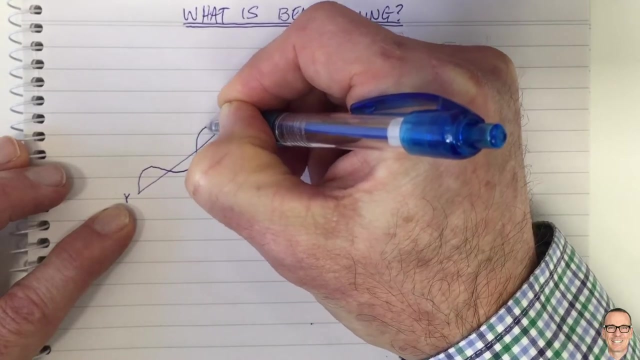 phone wireless communication signal, And so this is the path that it's coming in, on the straight line path to our receiver, And what's going to be happening is we have a waveform that is oscillating, So it's going in a sine wave as it comes towards us, because it's at a certain 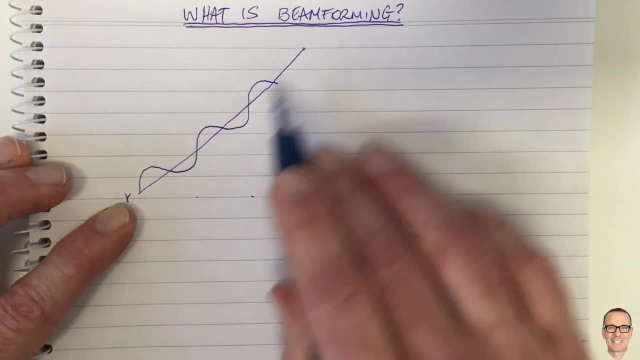 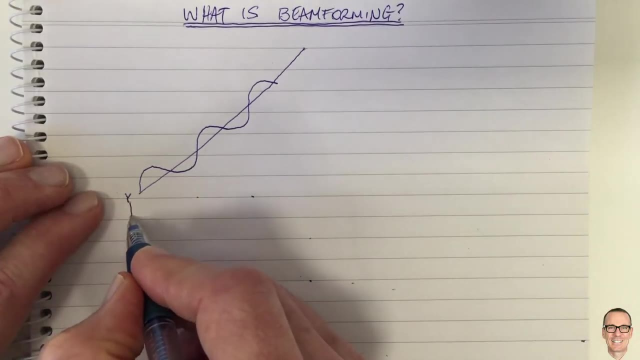 frequency. So this is a frequency that's coming towards us in a certain direction from that source. Okay, so what we're going to do is we're going to measure this signal and we're going to put this signal into our receiver, which is a bit of electronic circuitry. So I'm going to draw a box around our receiver. 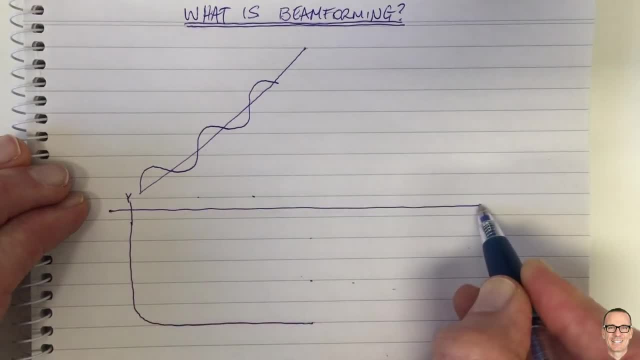 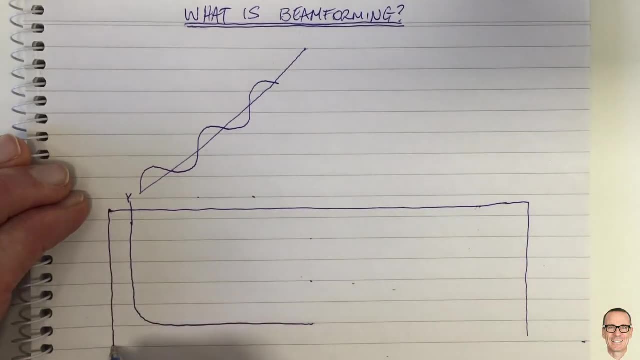 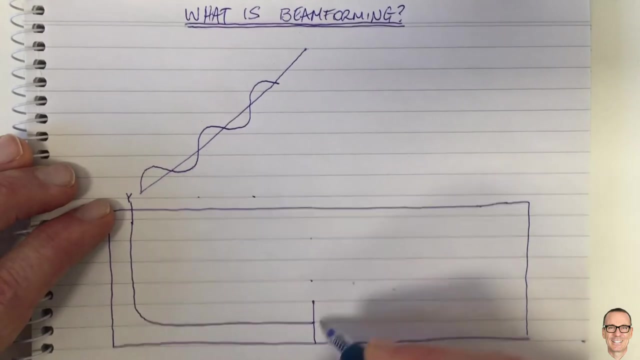 here, and so that we're really getting the idea that we are taking the signal into our signal processing unit. Okay, so we've measured the signal and what does it look like? Well, this signal here. it starts at zero and it's going in a sine wave, oscillating like this. So this is. 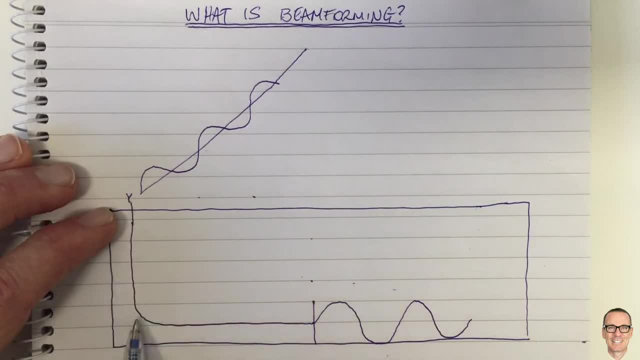 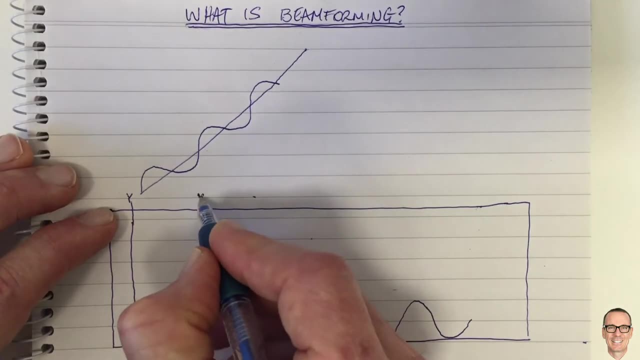 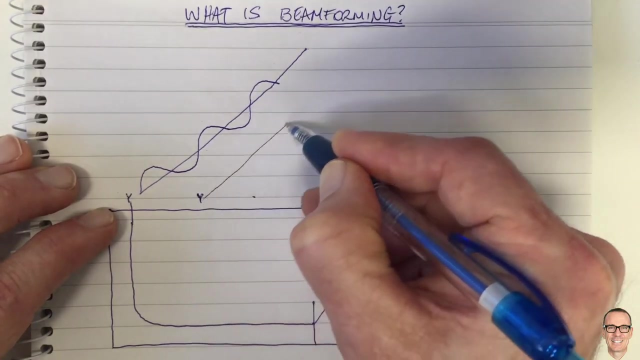 the signal we're receiving from our antenna into our electric wire and into our circuit. Okay, what if we had another antenna? So let's have another antenna here and let's think of our source as being so far away that it's coming in a parallel direction. So the source is a long way away. It. 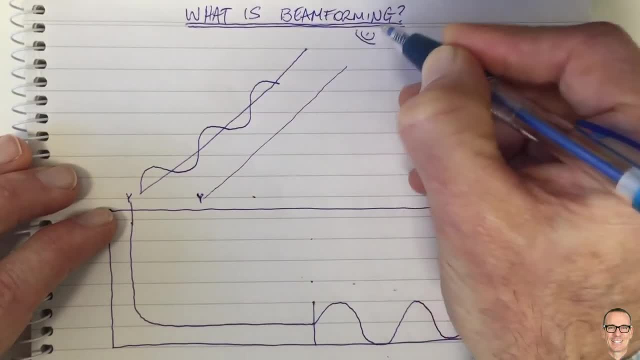 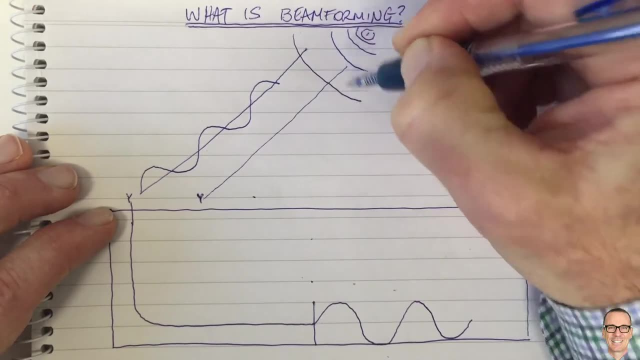 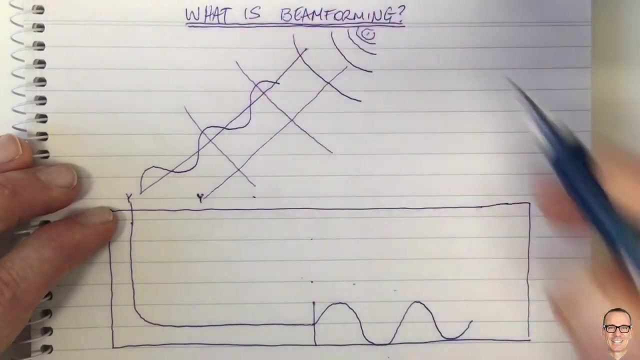 starts off emitting in a curve, of course radiating out from the source, But by the time it gets to us we are far enough away such that wherever these peaks are, they are straight line peaks. So the wave front is a straight line. We're going to assume a long distance away just for the moment. 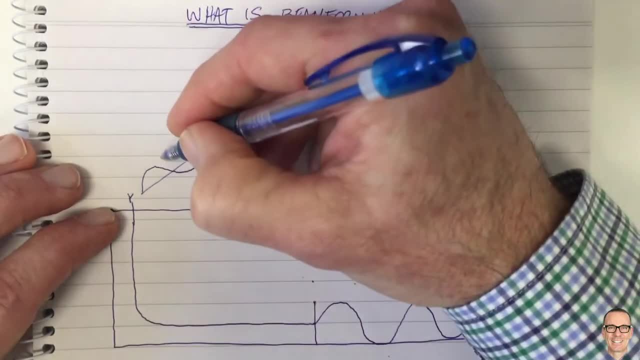 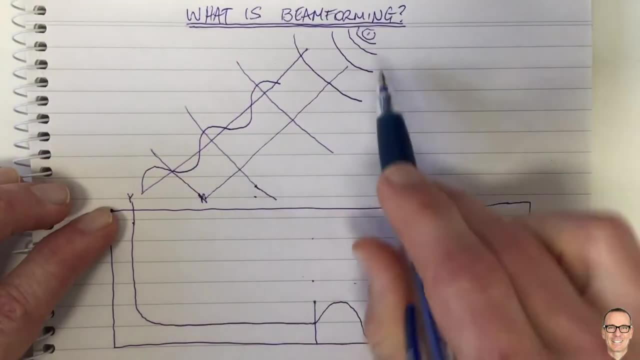 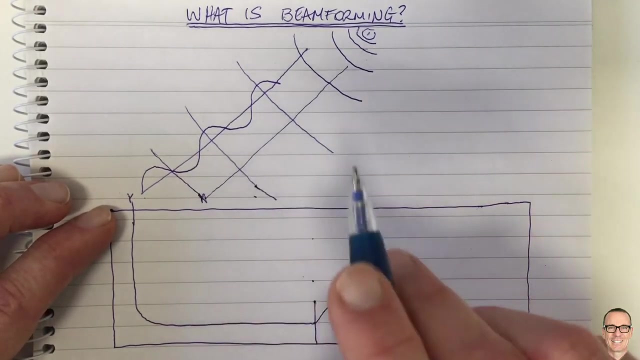 Okay, so what this shows us here is that this waveform, if it's coming from the direction I've drawn, it's going to reach this antenna first, Along this line. it reaches this antenna first, before it reaches this antenna, And the way I've drawn it, for this angle that I've drawn it and the frequency of wave that I've 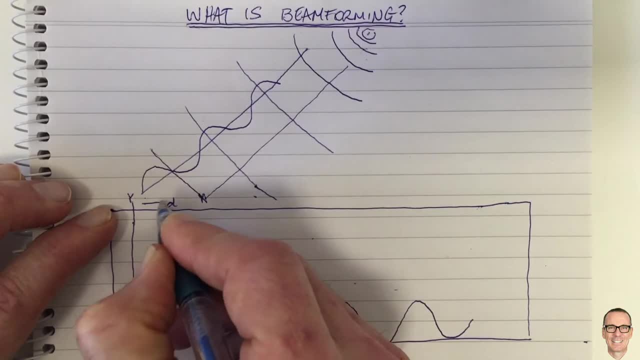 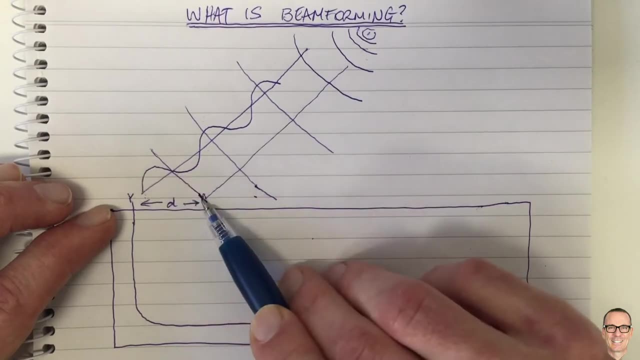 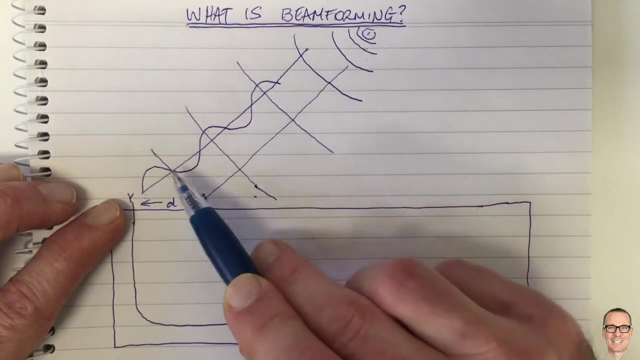 drawn, then, and the distance apart of these antenna elements, the way it's shown here, is well, it's going to arrive half of a wavelength here before it gets to this antenna. Okay, because this antenna is receiving this part of the wavelength but it still has to travel. that. 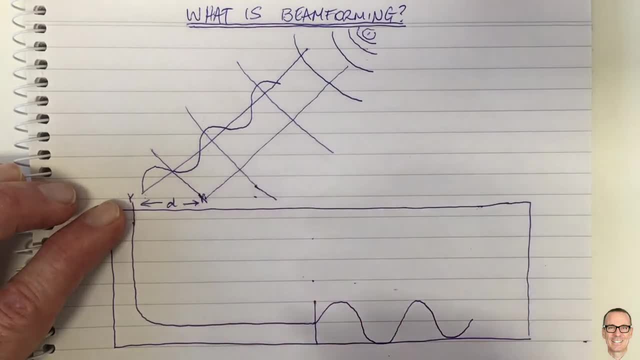 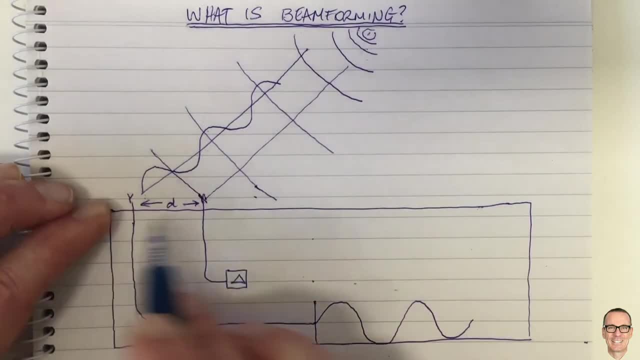 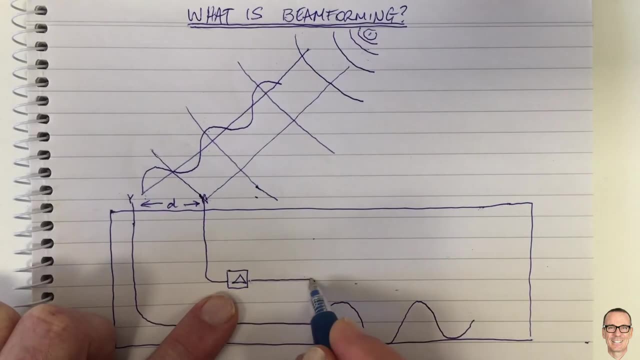 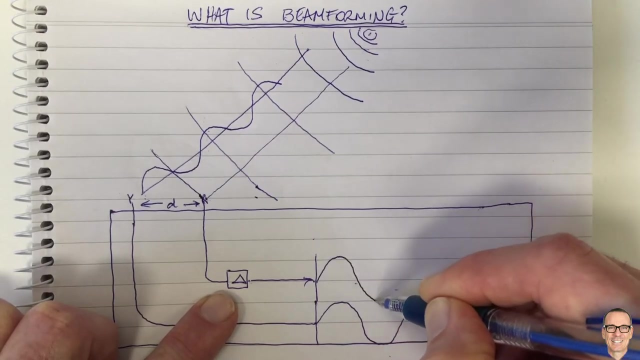 introduce a delay. So inside our electronics, in our sampler, in our electronics, we could do this in analog or digital. we're going to introduce a delay, And what's that going to do? Well, that's going to mean that these are going to line up in time, And so we can. then, if we've introduced that, 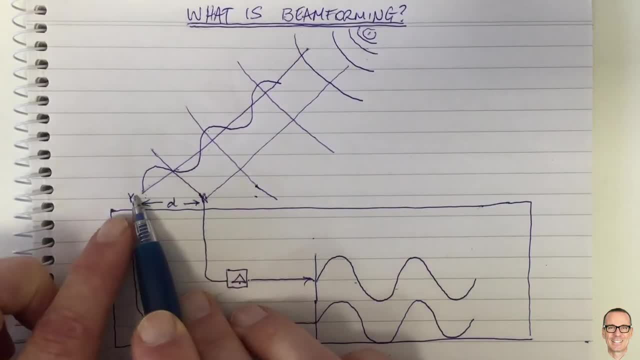 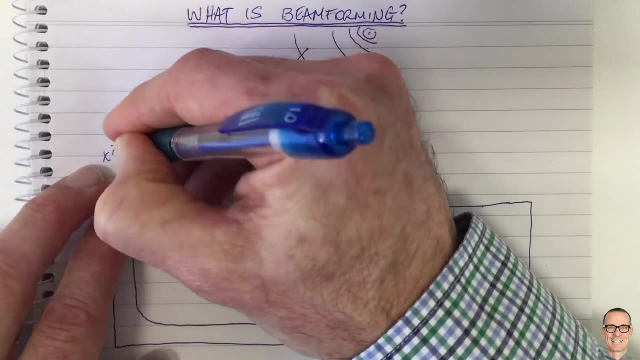 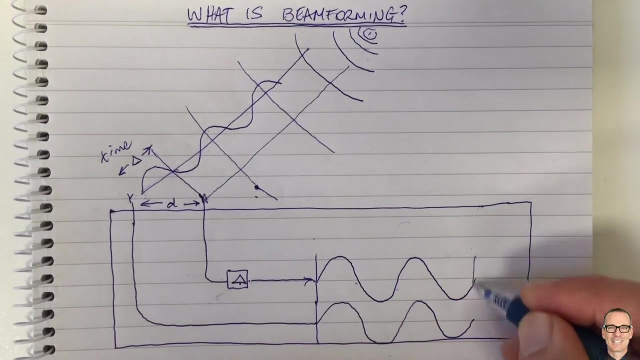 delay and if we've picked the right delay, which is exactly this time difference here. so this delay of time, that's a time delay, so this is time delay and this is a physical distance between the antennas. if you match those two up, then these waveforms will align and then we can put. 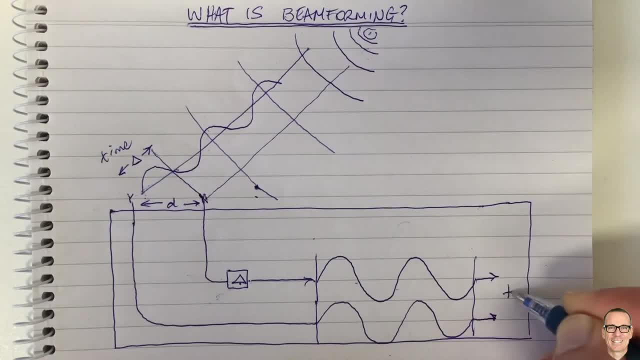 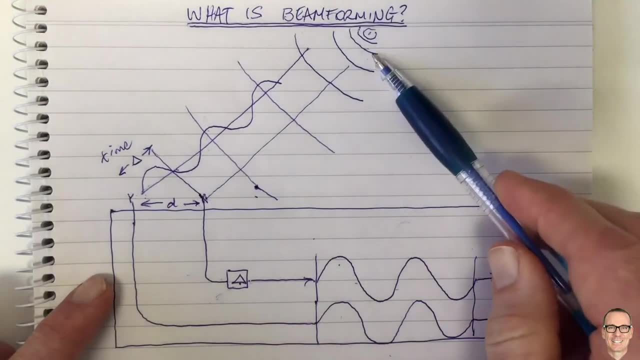 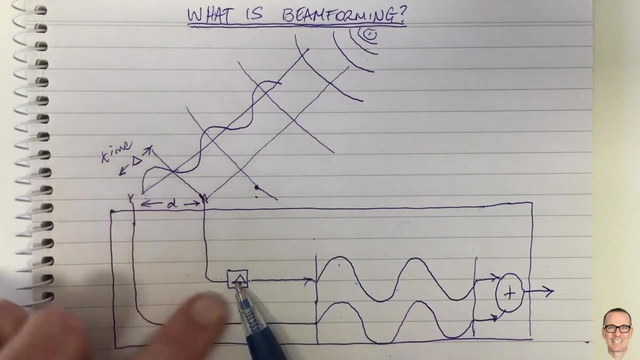 these waveforms into an adder and we can get a signal coming out which is the addition of those two. what it means is we're collecting more energy, so the energy from one antenna plus the energy from another antenna, and if we adjust the delay then they will add up in this way, where they their energies add and 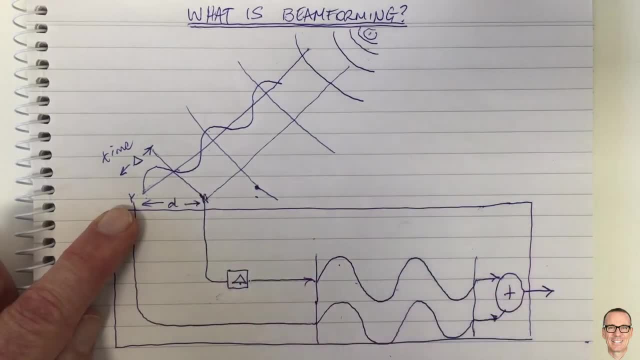 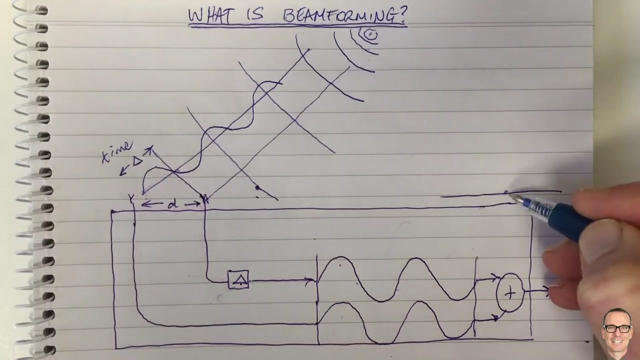 that's what we call beamforming. so why is it beamforming? well, we're getting the energy from that direction as an addition. so the two waveforms add. now let's think about this over here. well, maybe we're. I'm gonna plot a what we call it, a sort of a beam pattern. so in that direction, there we're getting a. 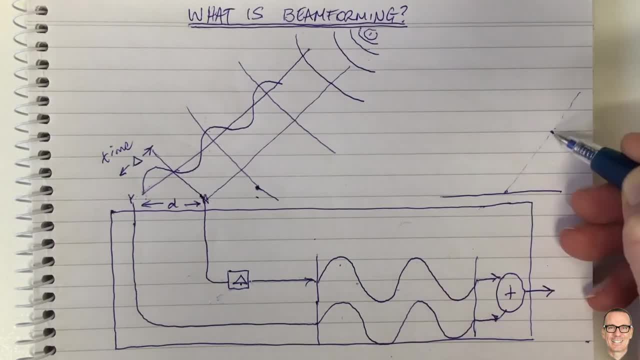 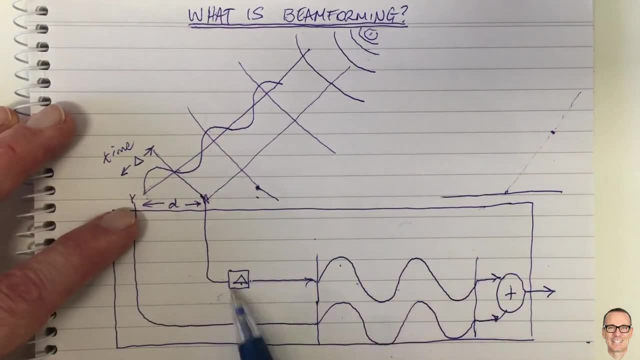 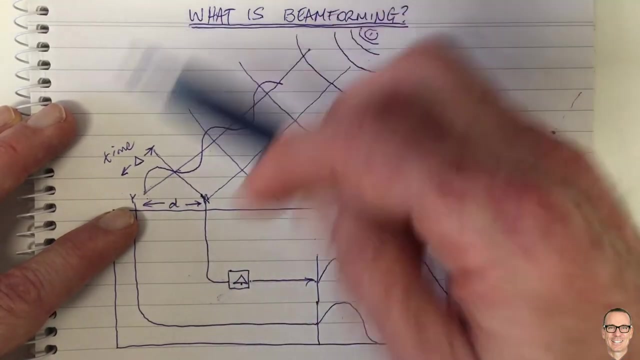 nice, strong signal. so if we think of the distance along this line as being the signal strength, we're getting a signal up here. well, let's think about the signal, another signal for the same delay, where we've tuned this delay to match that angle for this frequency in that distance. what about a signal from another user who's? 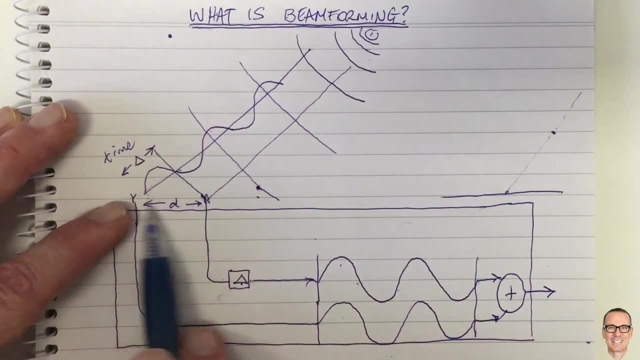 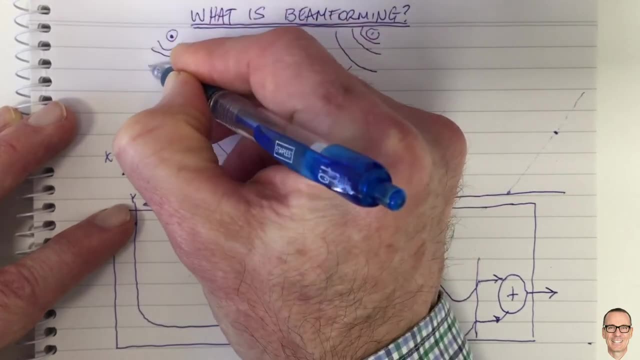 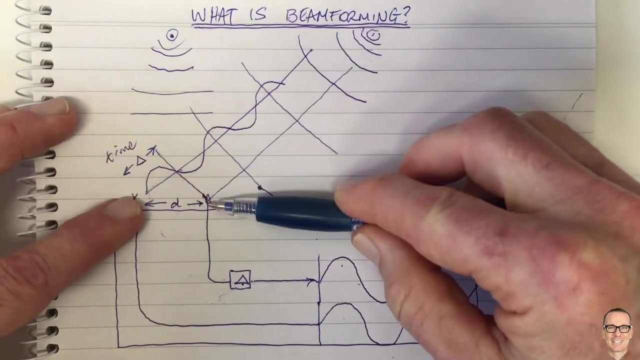 let's say straight off away from the antenna side on, so that waveform is going to arrive at our antenna again. we're going to assume it's a long way away, so that's going to arrive again with wavefronts which don't have any delay between them. so when our antennas, when 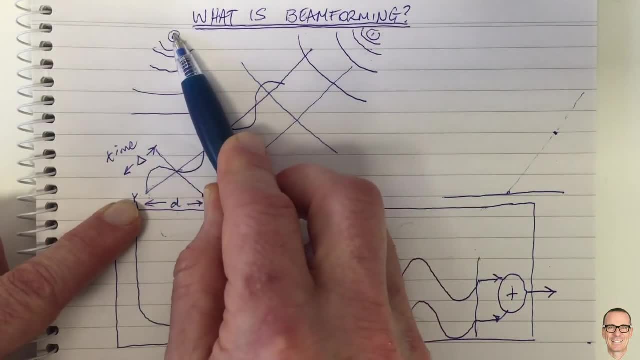 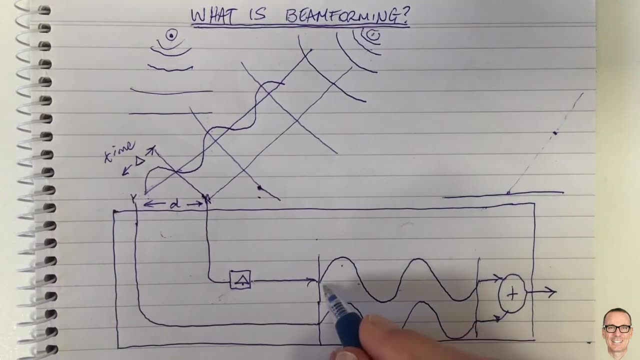 our two antennas receive them and there's no delay for this source, at this direction, there's no delay. but we introduce a delay and we're introducing a delay of half a wavelength. well, we're going to get this. one's going to come through straight as a signal like this, but this one is going to come through. 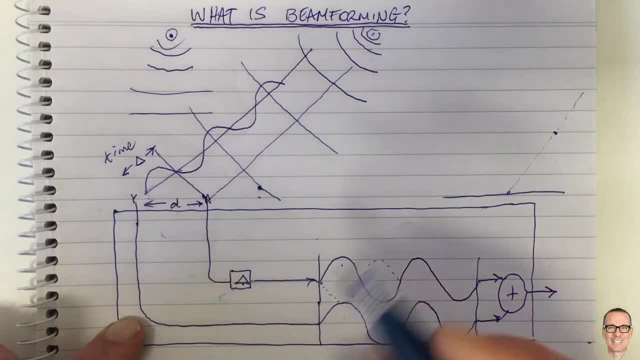 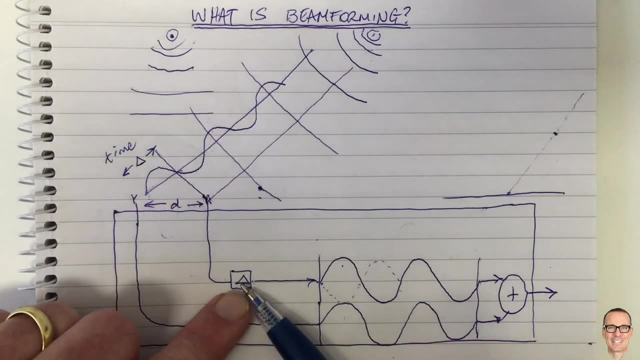 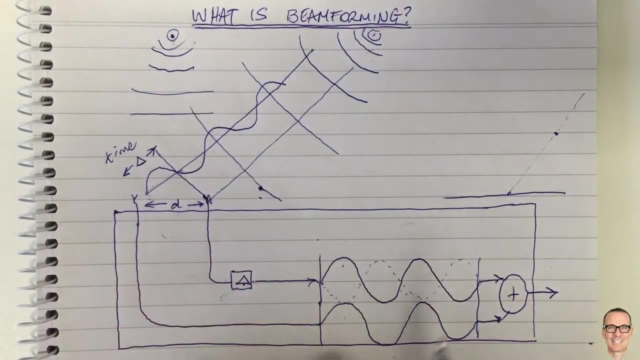 exactly half a wavelength out because there was no delay from the physical situation of the wave fronts hitting us. but we've introduced a delay So for signals coming from this direction they will add up exactly opposite each other and cancel each other out. So the one coming through here with no delay, this: 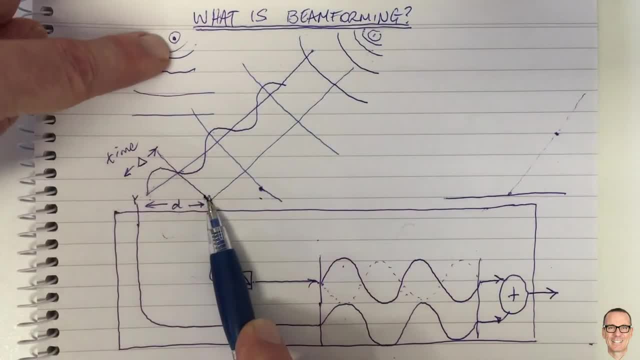 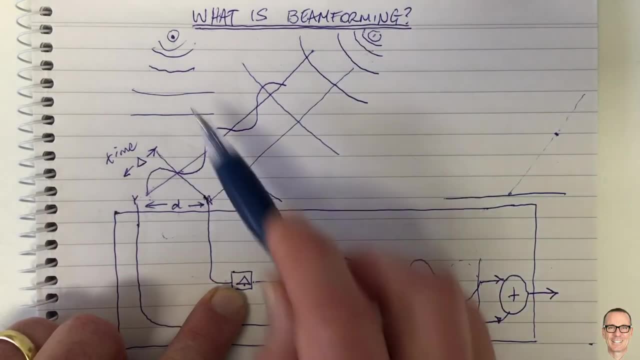 will be the normal waveform, The one that's coming through from this antenna, from that transmitter, is going to be. we're introducing a delay because we've tuned it for this direction and it's now it for this direction is going to exactly cancel and we'll get zero coming out. So in the, in the direction, 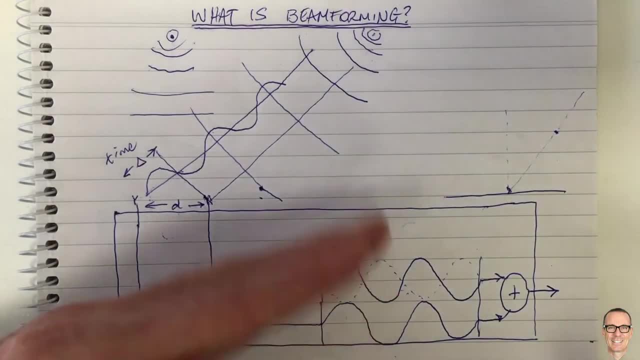 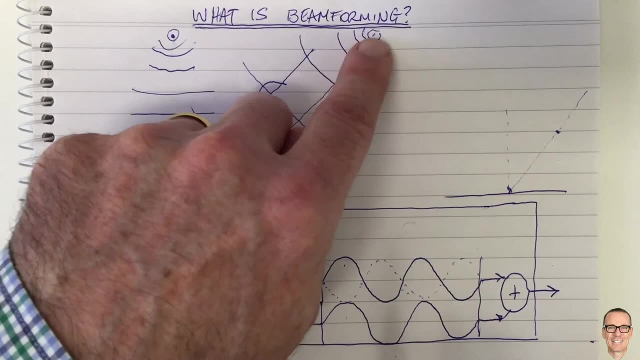 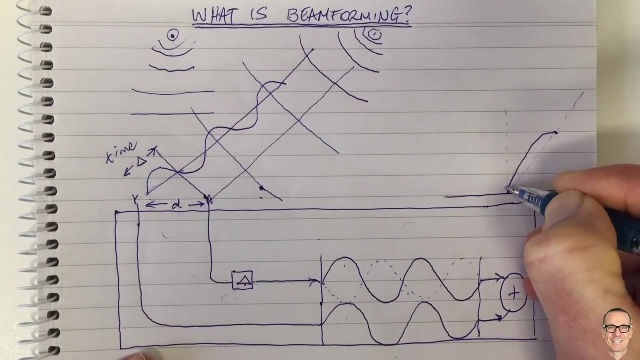 straight off. we're getting actually zero and you can think, you can imagine as we swift around. if we keep this delay fixed in our processing, if the, if the user, the transmitter, if the transmitter moves around, then we'll be getting different signal strengths from that transmitter and they'll be forming. 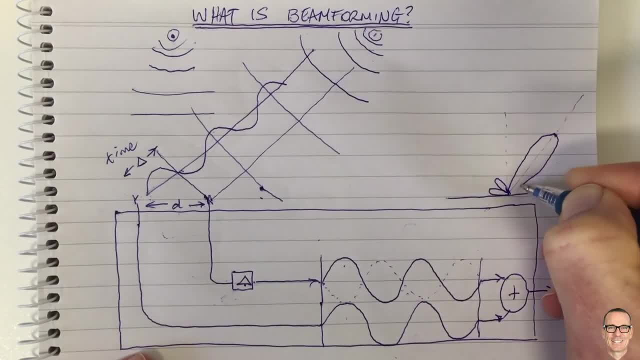 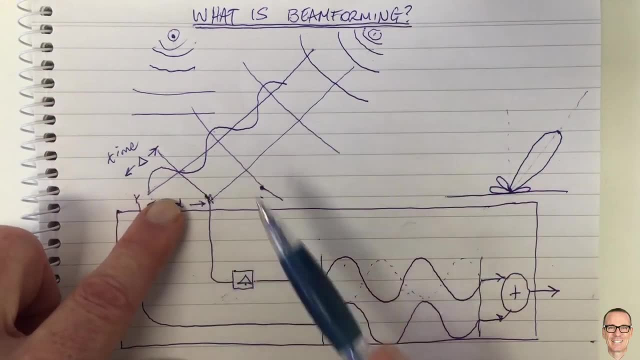 something that we call a beam and it's going to have different, different angles. they will add together and at other angles they will cancel. this way, angle like this Canceled for this scenario, this angle they added perfectly and we got a good, strong signal and this is what we call a beam pattern and this is called beam. 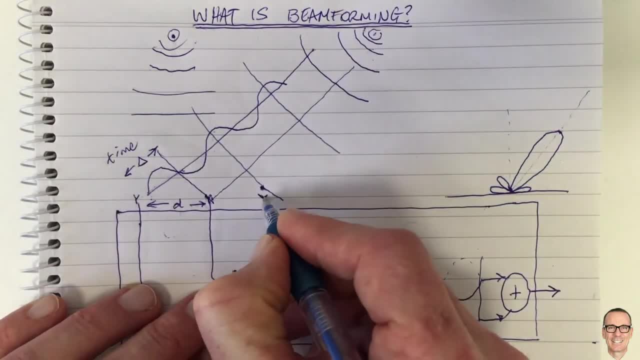 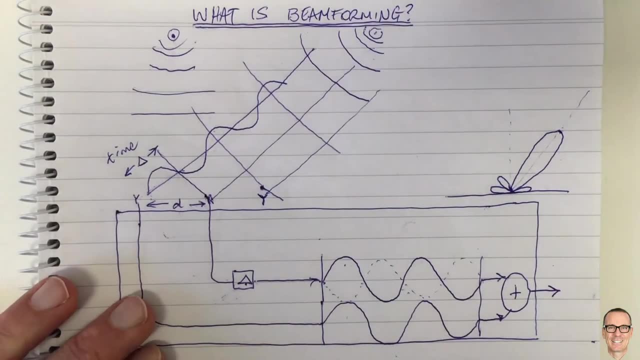 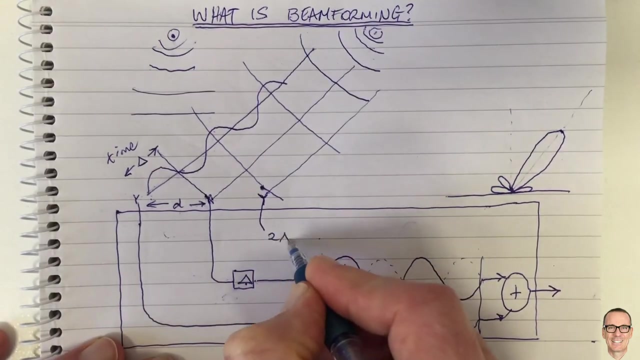 forming, Of course, if we had a third antenna here. so we're collecting even more energy, and it's always good to collect more energy, especially in signals that are weak and there's lots of noise. so we want to have lots of collection of energy For this one. we could add two times the delay if we're.